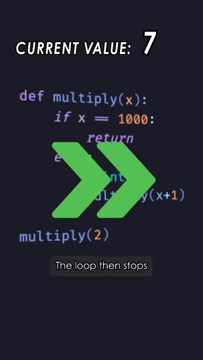 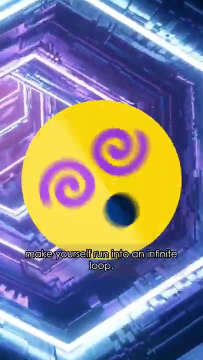 1000.. I rely on the current value in the current loop. The loop then stops when the condition is met. However, make sure that when actually happens, because you can accidentally make yourself run into an infinite loop, An infinite loop. 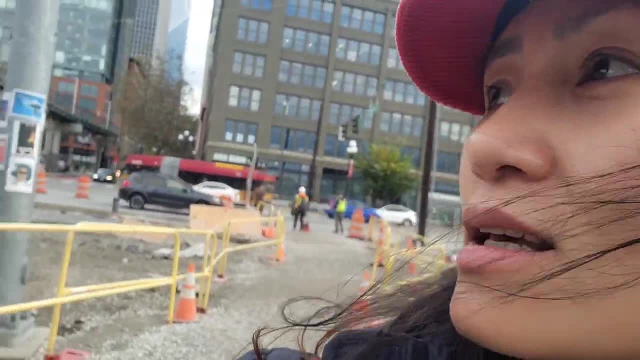 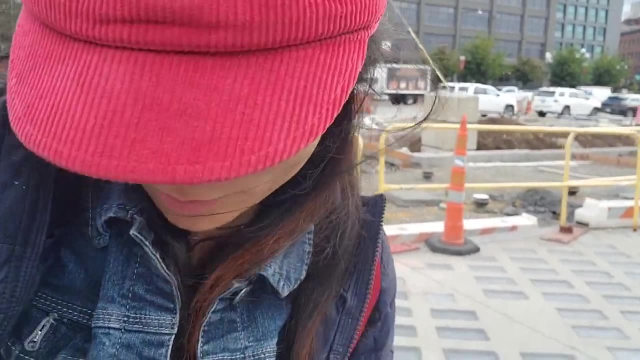 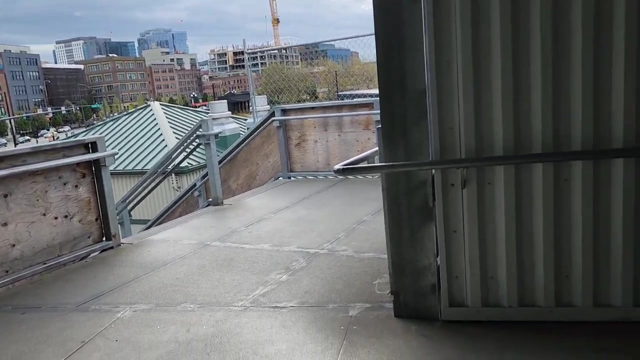 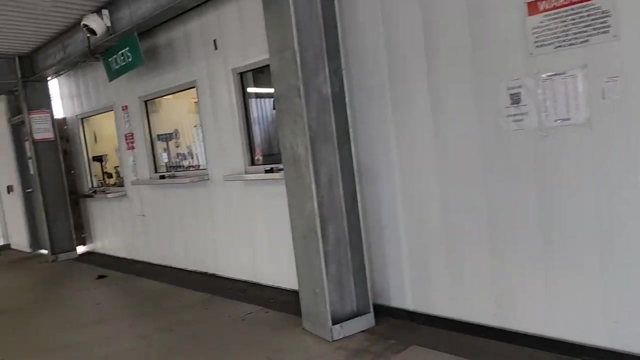 So I'm back in Alaskan Way, About to go find my way to the ferry. This time I'm using a different ferry. I just climbed up stairs- Whew, hit my back. Good thing it's not too heavy. Now I'm going to buy ticket. 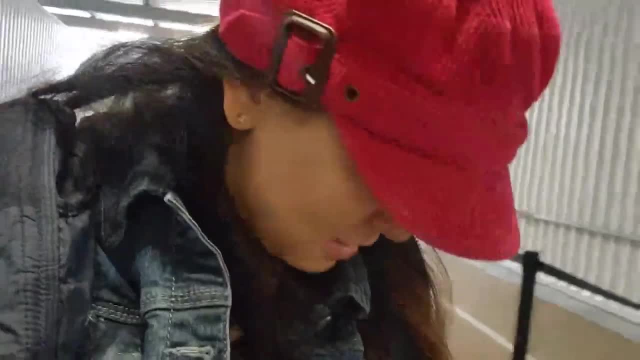 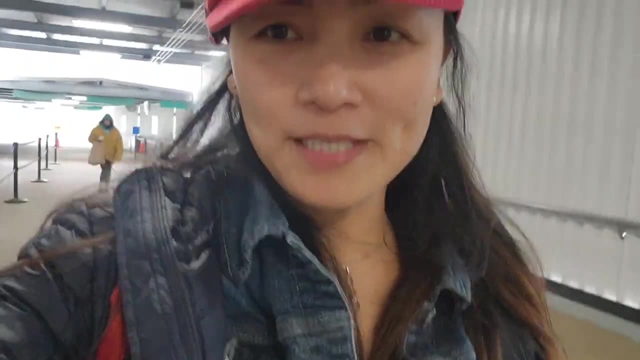 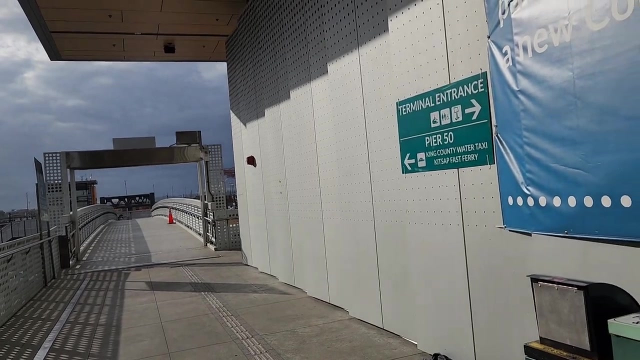 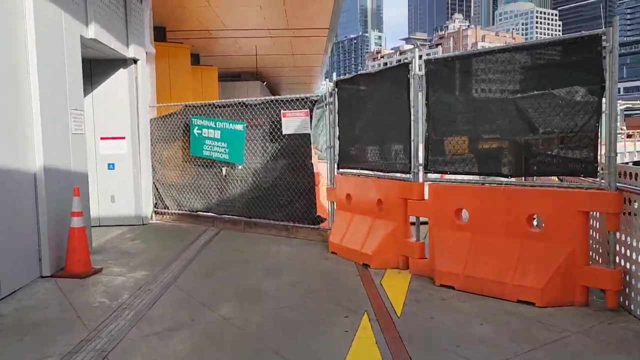 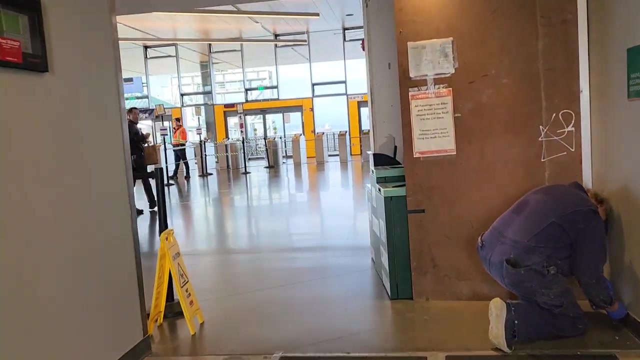 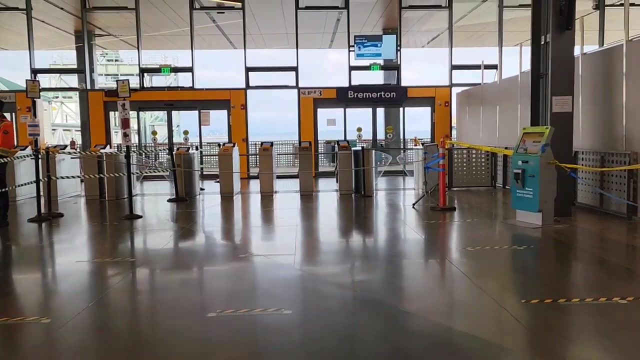 The ferry won't leave until 12.40 something, So I have time That there is going to Pier 50.. I'm going this way. There's some work. I'm going this way. See, Bremerton is right there, But the time 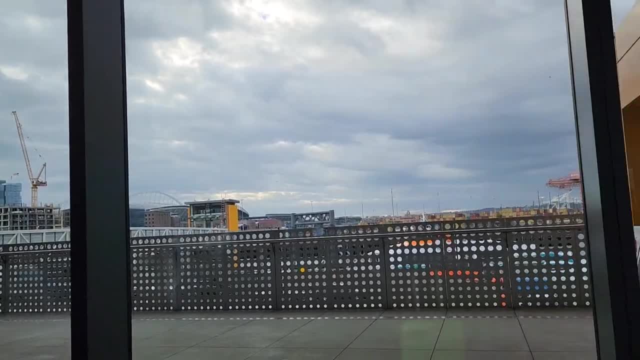 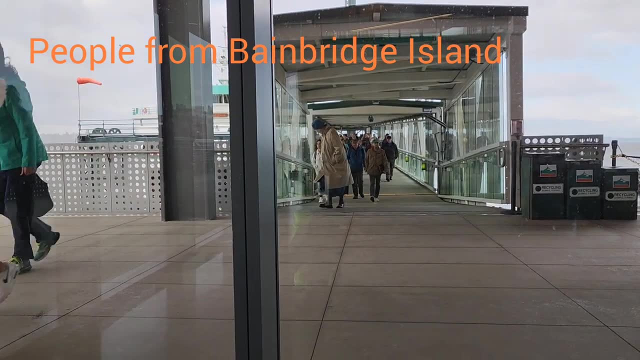 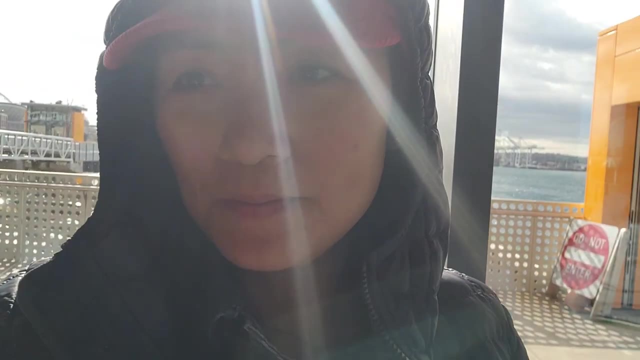 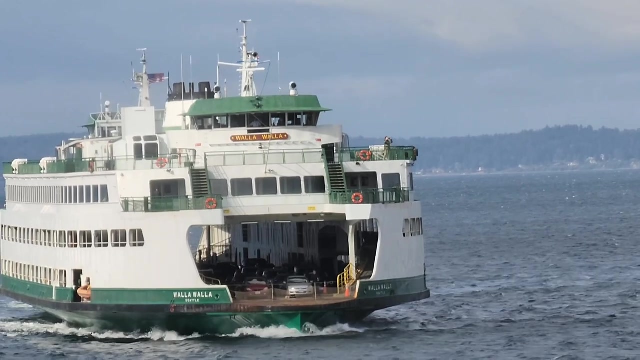 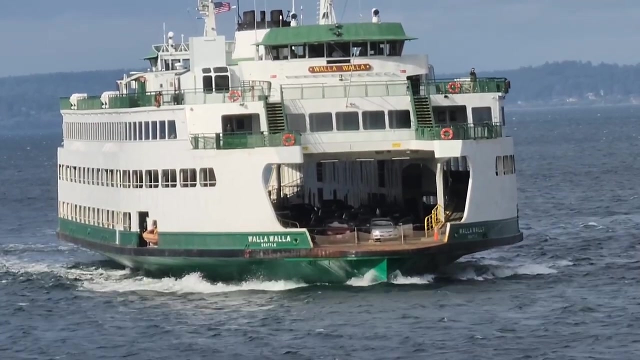 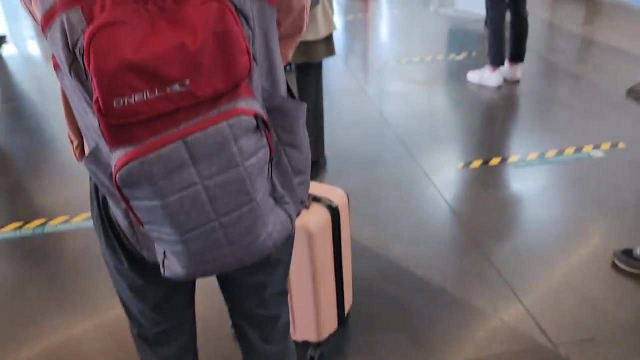 Windy and cold in Seattle. People just un-shines. It's a bit cold inside here, So I believe that is our ferry Walla Walla. It's 9.45.. Cash Inside 9.45.- 9.45..